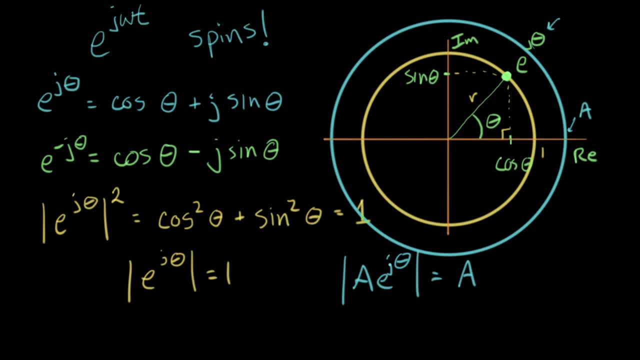 In the last video we did a quick review of the exponential and what it means, and then we looked and figured out what the magnitude of an exponential is. The magnitude is equal to one. Now we're gonna look closely at this complex exponential, as it represents a cosine, a part of a cosine. 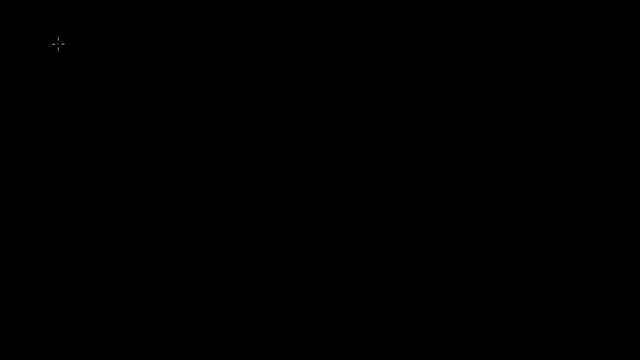 Now we're gonna keep combining some of our ideas from the last couple of videos And you remember, one of the things we did was we used Euler's formula and turned it inside out and developed an expression for cosine. So if I say cosine of theta, 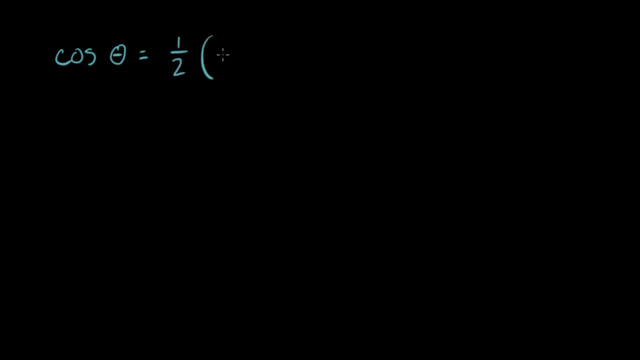 I can say that equals 1 1⁄2 times e to the plus j theta, plus e to the minus j theta. This is cosine of theta expressed as two separate exponentials. And now we're gonna take a really special step. I'm gonna put in an argument right here of time. 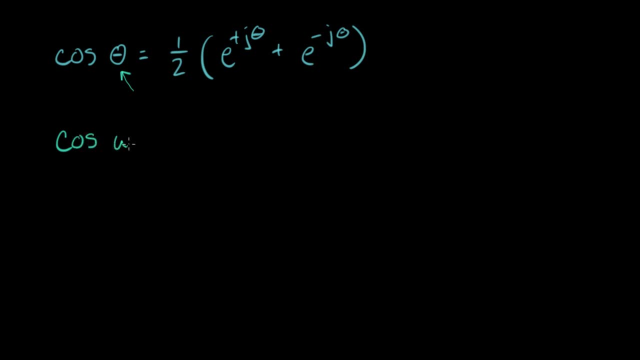 I'm gonna say cosine of omega t. T is time and this shape here, this symbol here is the lowercase omega from the Greek alphabet and that's the frequency. So time is in units of seconds and omega is a frequency, So it's in units of one over seconds. 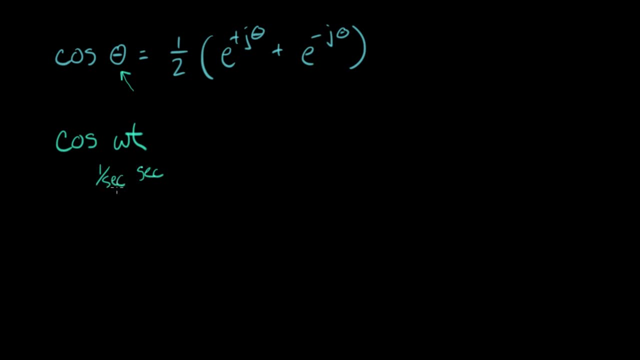 That's the units of frequency, It's a frequency or per seconds, And when these multiply together we get dimensionless number right here, and we can take the cosine of a dimensionless number. So what does this equal to? This equals 1 1⁄2 times e to the plus j, omega, t. 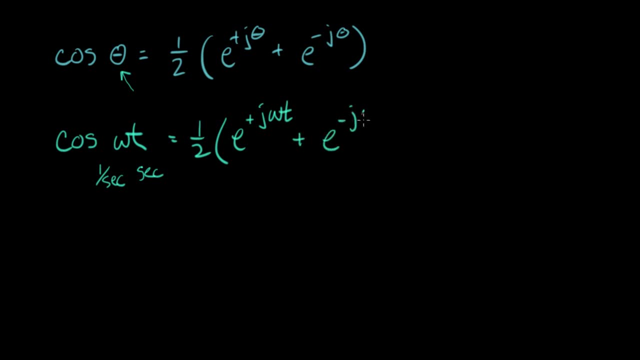 plus e to the minus j, omega t, When we make t the argument of the cosine here. t is the stuff that keeps going up and up and up. The number t just gets bigger all the time, And so we ended up with a cosine wave form. 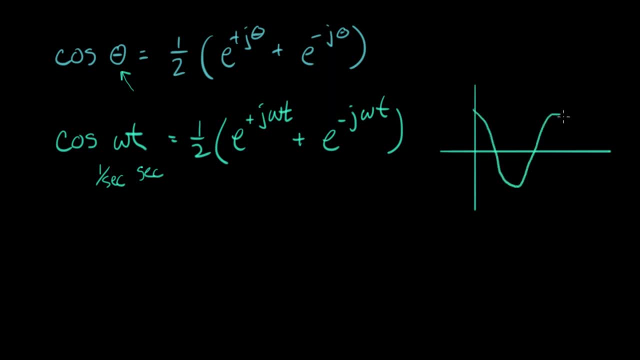 and I'll just make a bad cosine-looking thing here. That's what a cosine looks like, and it keeps going and going and going. So we have an idea of what a cosine wave looks like. The frequency determines how fast this goes up and down. 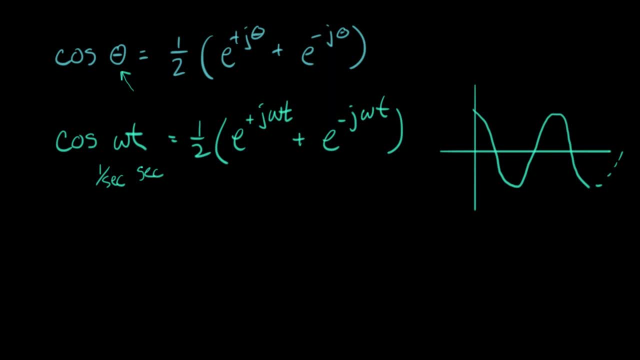 or how often it goes up and down. But now what I wanna do is I wanna look at a really special thing. I wanna look at what is the frequency? What is this thing right here? What is this thing? e to the plus j, omega t. 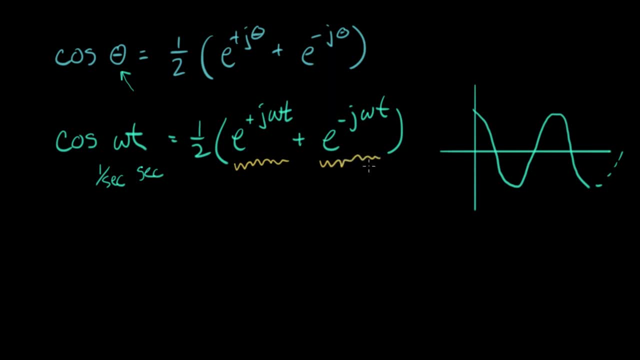 And what we see is this cosine here is made of two of these things. So whatever these things are, I can make a cosine out of them. So now we're gonna look really carefully at e to the j, omega t. What we just reviewed was that this is a complex number. 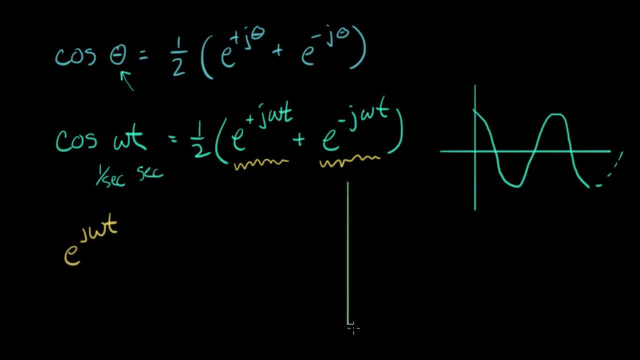 Let's draw that complex number. We said that that goes under the first aumentant of t. Here's my new number, So we're gonna put our number out here. We know it falls on the unit circle, We know its angle. So this angle right here is omega t. 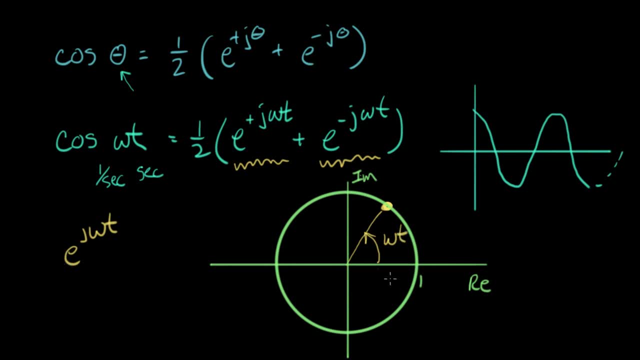 And we know the magnitude of this is as we decided before. the magnitude is one. That's why it falls on the unit circle. Okay, so now look at this. Here's this number: t that's determining the angle, And that means what? 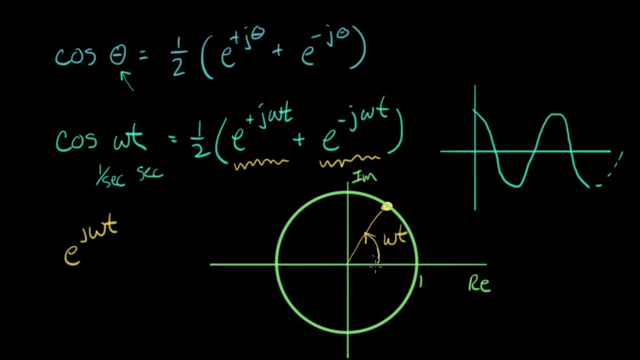 That means that the angle is increasing with time. If time is equal to zero, the point is right here. at time equals zero, Because angle is zero. As time proceeds, the angle starts growing and growing And it basically keeps growing and it keeps going. 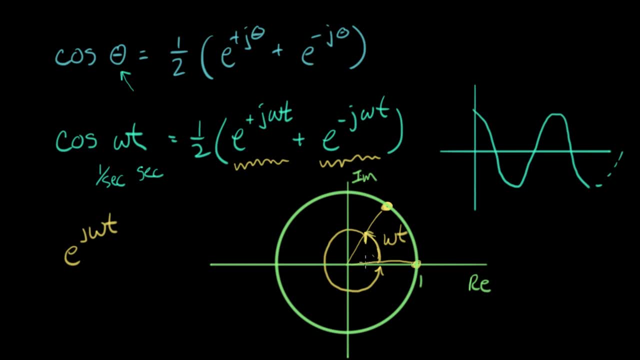 It comes back to here after omega t equals two pi. And then what happens? It keeps going around it again, And this basically goes along for as long as time goes along. So here's this number, Here's this complex number moving along the unit circle in time. 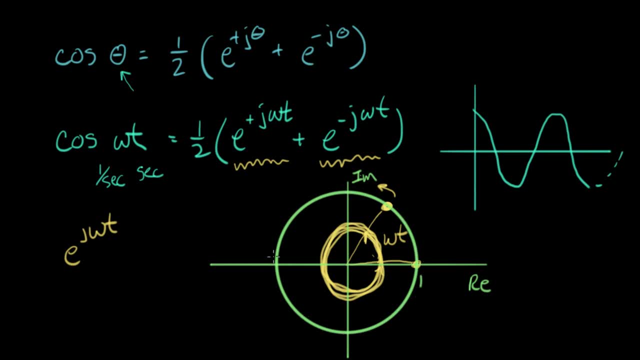 over and, over and over again. So this is a number that is rotating. The number is rotating So I can write here e to the j, omega t, And I know that that because time's up here, I know it's rotating in time. 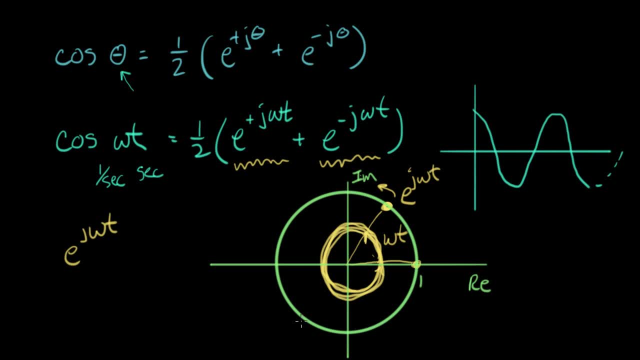 Alright, now I'm gonna put a different number on there. Let's put it over here: say: Well, let's actually start this number at zero And I'm gonna call this number e to the minus j, omega, t. What does that number look like?